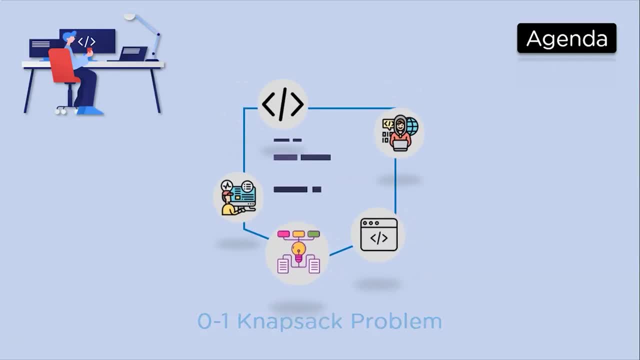 and discuss the zero-one knapsack problem. After that we will look into its implementation in the code editor. Then we will discuss the fractional knapsack problem. Finally, we will dive into its implementation in the code editor. But before we begin, make sure you have subscribed. 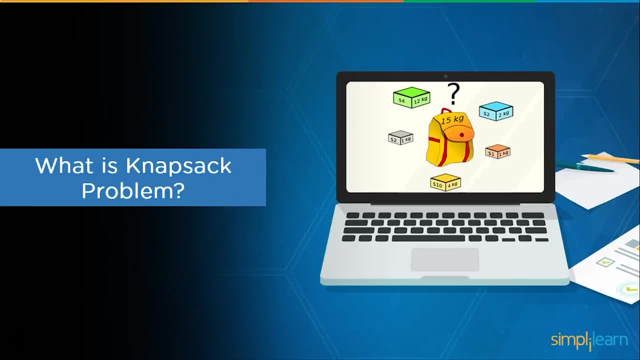 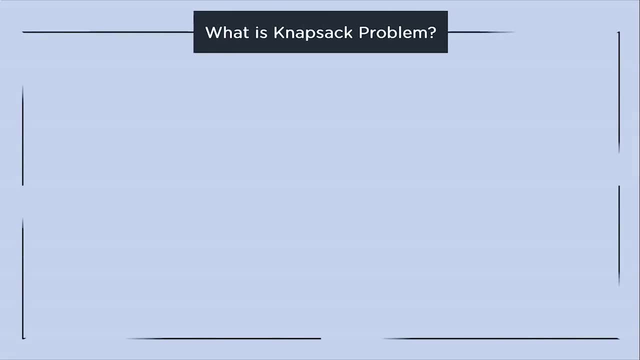 to our YouTube channel and clicked on the bell icon below So you never miss an update from Simply Learn's YouTube channel. So, without any further ado, let's get started. Let's get started with the topic. what is knapsack problem? 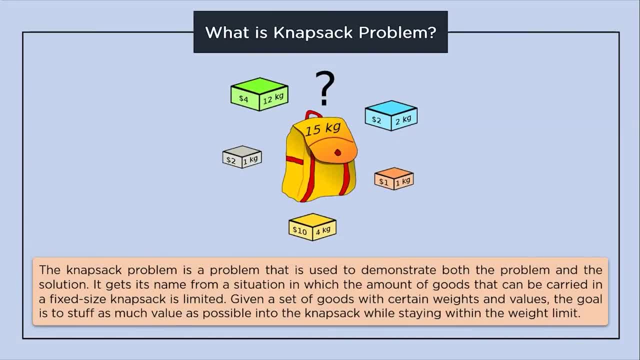 The knapsack problem is used to explain both the problem and the solution. It derives its name from the fact that the limited number of things that may be carried in a fixed-size knapsack Given a set of items with varying weights and values. the goal is to pack as 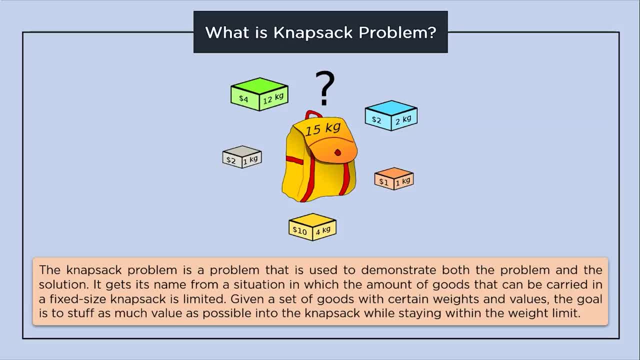 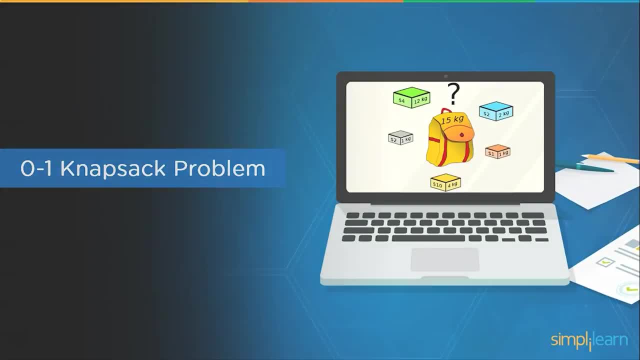 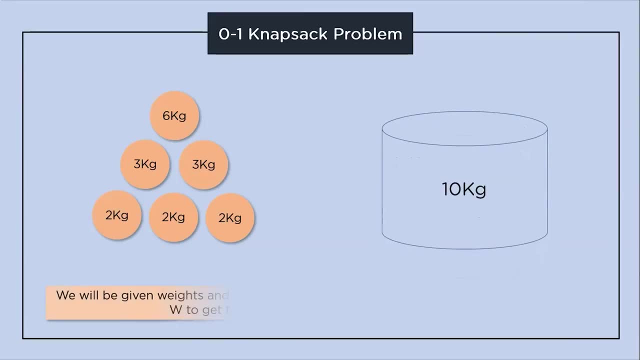 much as value as possible into the knapsack while staying within the weight limit. Now let's discuss zero-one knapsack problem First. we will be given weights and values of n items, In this case 6 items on the left. We will put these items in a knapsack of capacity. 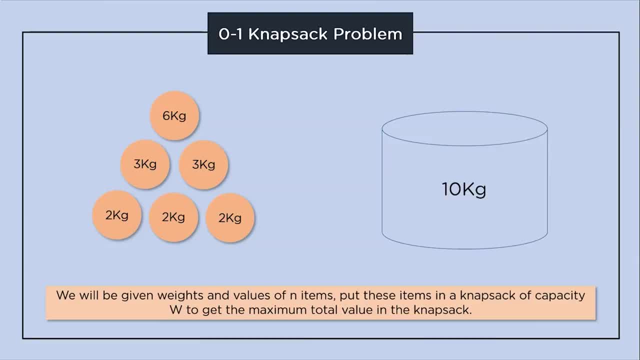 or in this case 10 kgs, to get the maximum total value in the knapsack. Then we will have to fill this knapsack but we can't break the item. So we must either pick the entire item or not pick at all. due to this, sometimes it may even lead to a knapsack with some spare space. 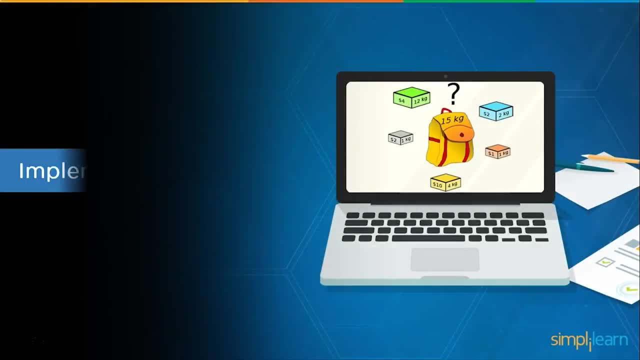 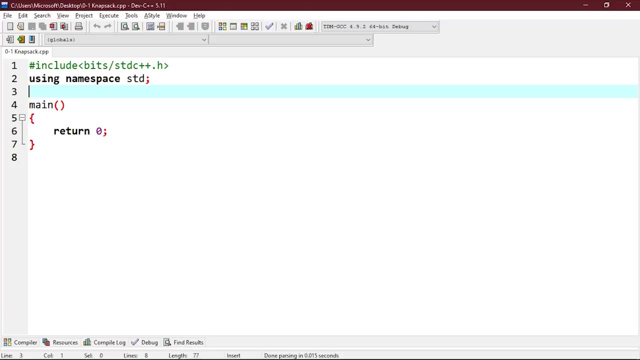 left with it. now let's try to implement this in the code editor. we will start with the utility function that will return the maximum of two integer int: max, a, comma and b. we will return. if a is greater than b, then a else b. we will now write a function to return the maximum value that can be put in a knapsack. 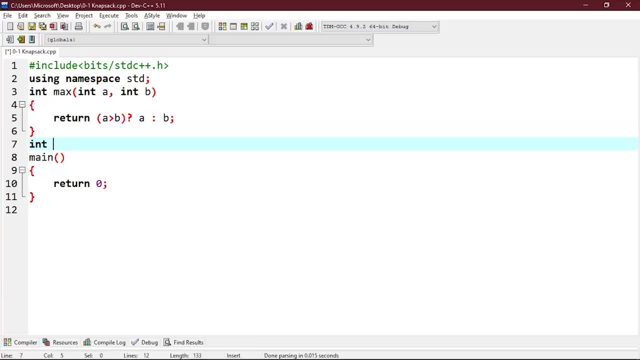 of capacity w int, knapsack int capital w comma int wt for the weight comma int, value comma int n d. we will declare int i w. we will create a vector inside a vector a n plus 1, comma, vector int. 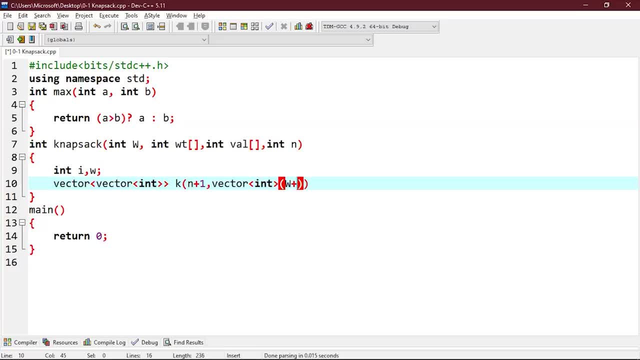 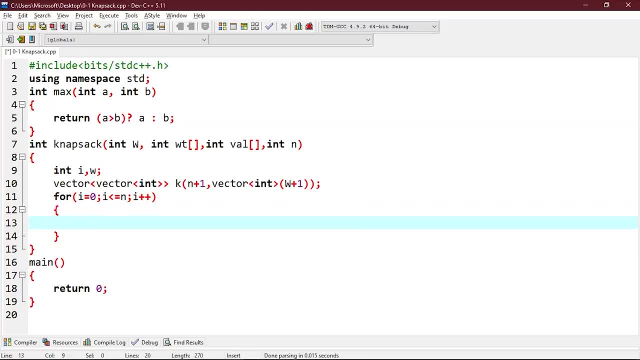 W, we will have another for loop inside it, for loop with small w equals to 0,. this small w will be less than equals to capital W, with small w plus plus. Now, if i is equals to 0, or W is equals to 0,, then we will have k i comma W. 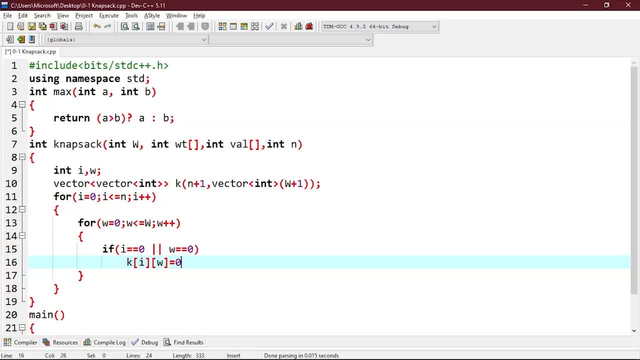 is equals to 0, else if weight at i minus 1, is less than equals to W, then we will have k- i minus 1,. then k at i comma W will be equals to max of value at i minus 1,. 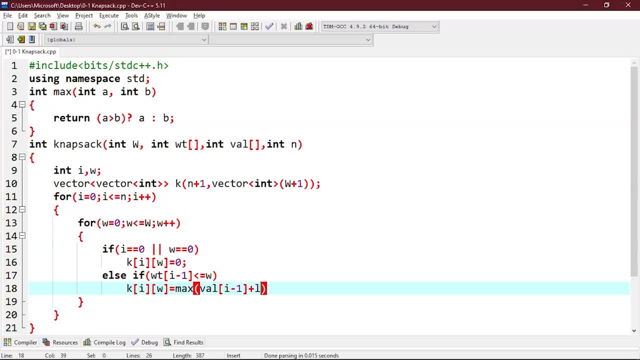 plus k at i minus 1, comma W minus Wt, where Wt is at i minus 1, plus k at i minus 1, comma A, at i minus 1, comma W. else, 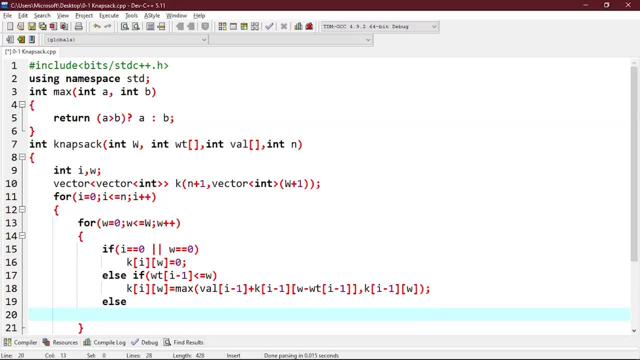 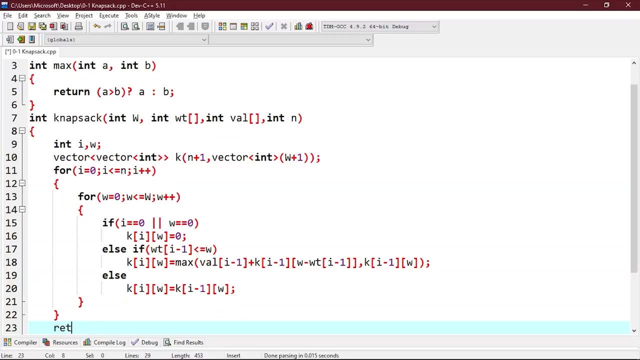 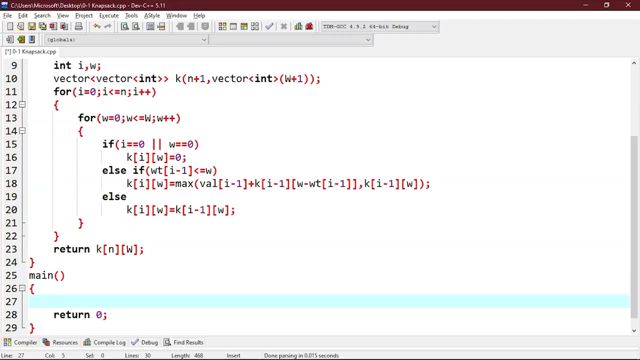 We will have k at i comma w is equals to k at i minus 1 comma w. Now we will return k at n comma w. Now we will write the main block. We will start with int value at i comma w, Int value array, which will have elements as 60 comma, 100 comma, 120 and weight will. 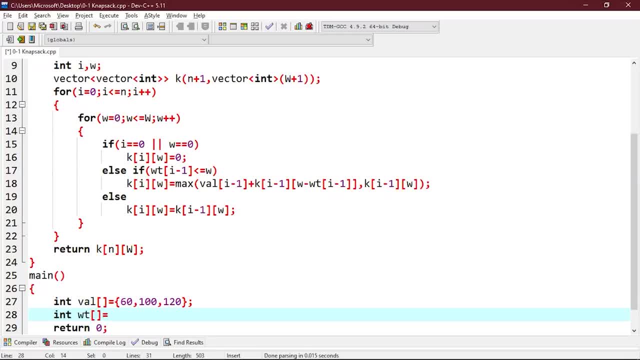 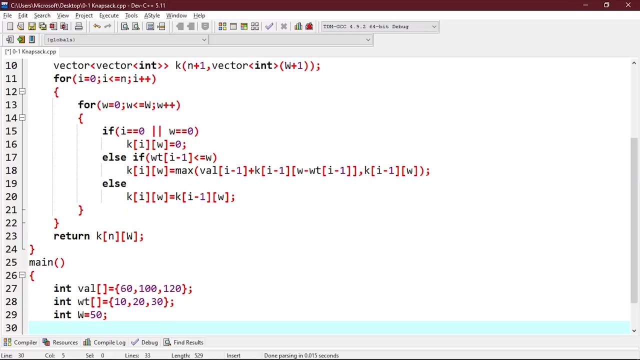 be equals to 10 comma, 20, comma, 30. And the maximum capacity, the capital W, will be equals to 50.. Now let's find the size of the value array. So int n is equals to 50.. Now let's find the size of the value array. 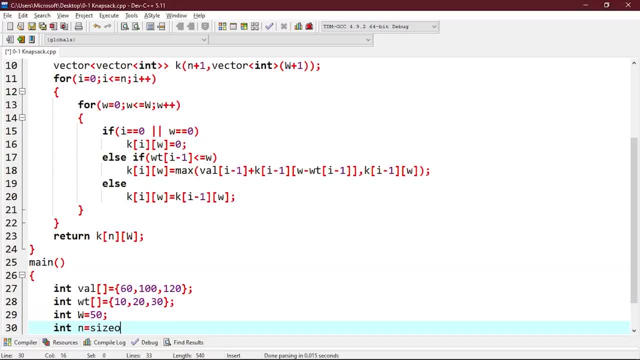 So int n is equals to 50.. Now let's find the size of the value array S. MY dot保 chocolat is equal to 60 comma 10 comma 20 comma 95. And the maximum capacity, the capital W, in this case, is 60 comma 10.. 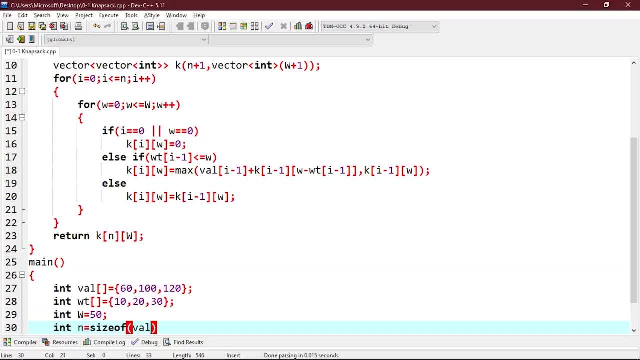 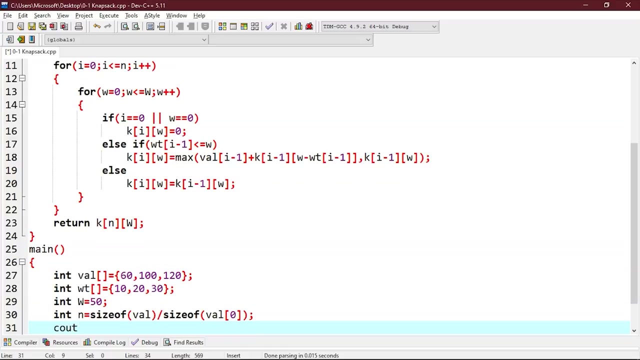 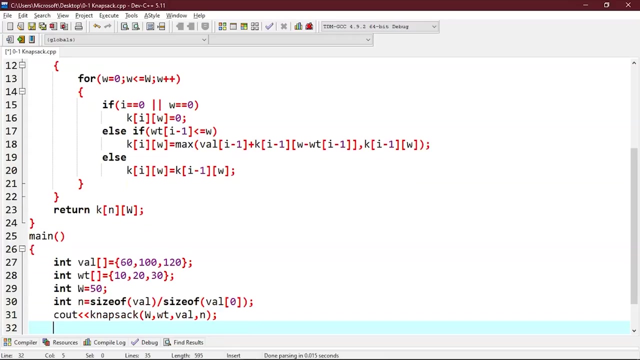 And the maximum Pacific FLовать was equal to 50 comma 10 comma, 22 comma 75.. And the maximum capacity the capital PP quot was equal to can also be equal to on sizeof cout knapsack at capital W comma, WT comma, val comma n and return it as 0. 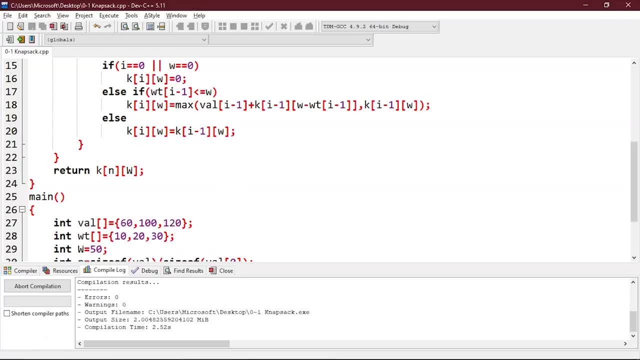 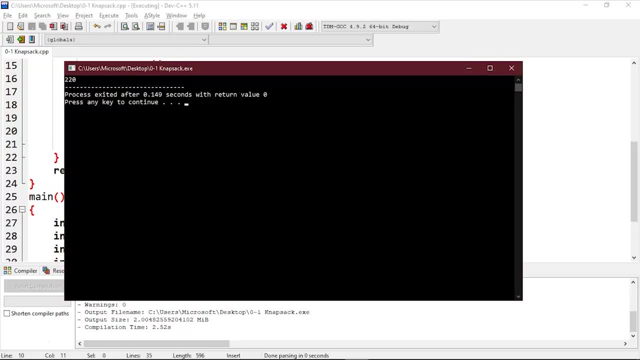 let's compile it. as you can see, we are getting the value as 220, which means we are getting it because we are taking the elements with weight equals to 20 and 30, which comes out to be as 50. let's get back to our slides. if getting your 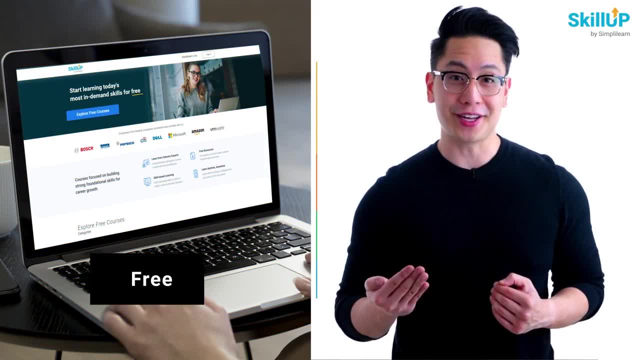 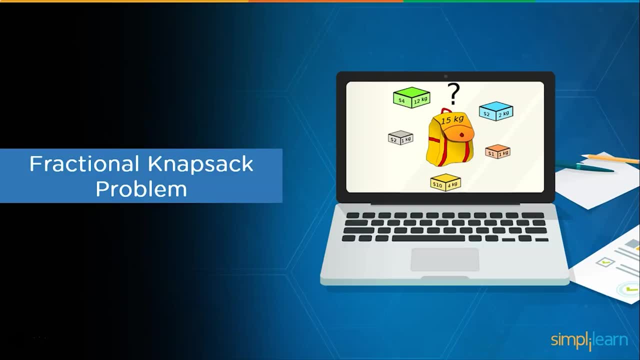 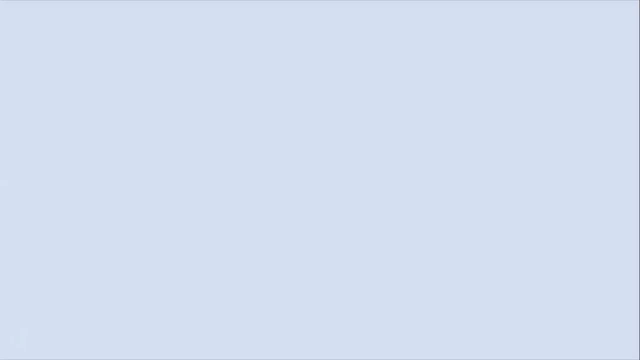 learning started is half the battle. what if you could do that for free? visit skill up by simply learn. click on the link in the description to know more. we have now discussed 0- 1 knapsack problem. now let's discuss the fractional knapsack problem, similar to: 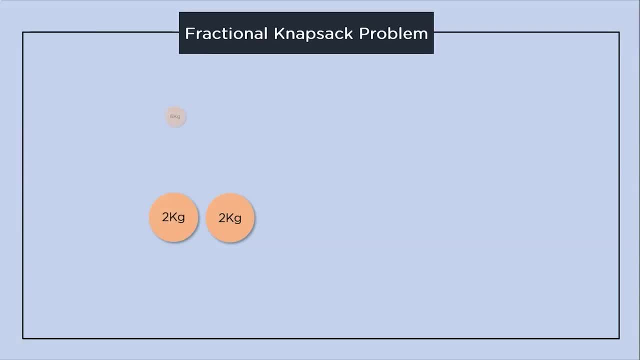 the 0- 1 knapsack problem. we will be given the weights and the value of n items, in this case 6 items. on the left, we will also be getting a knapsack with capacity W or in our case, 10 kgs. to the right, 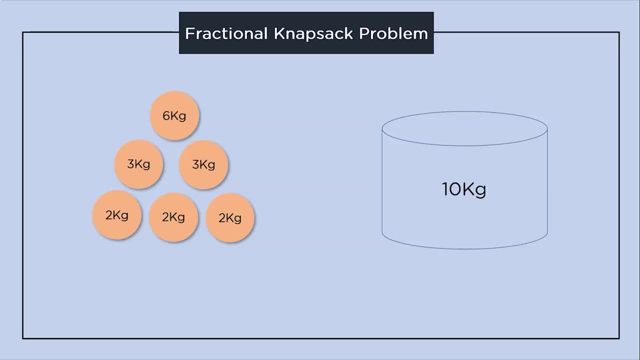 now we have discussed the fractional knapsack problem. now let's discuss the 0- 1 knapsack problem. now we have to get the maximum total value in the knapsack. then we will have to keep filling this knapsack but, unlike 0- 1 knapsack, we can. 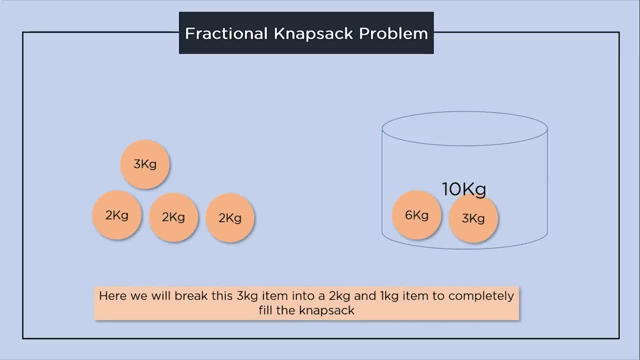 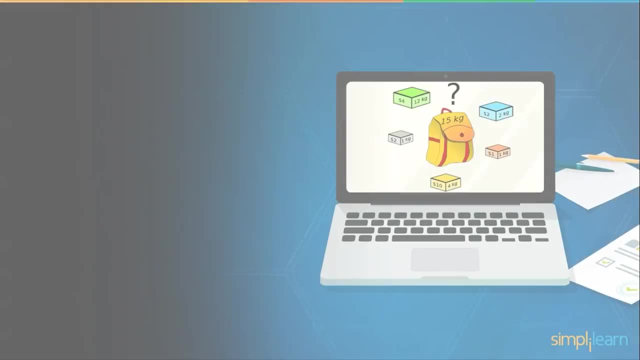 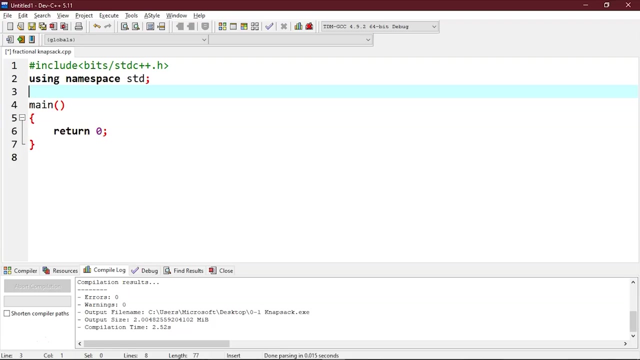 break an item to get a maximum value of knapsack. here we will break this 3 kg item into a 2 kg and 1 kg item to fill the knapsack. now let's try to implement this in the code editor. we will start with the structure for an item which stores weight and 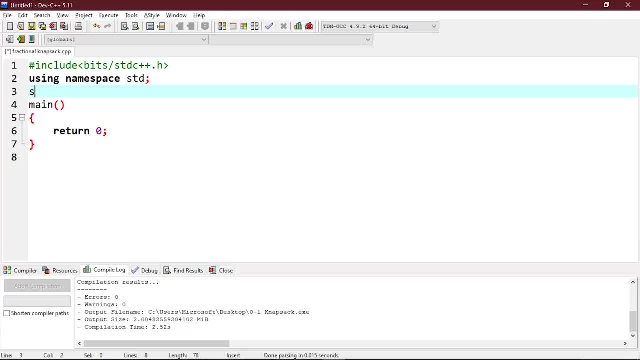 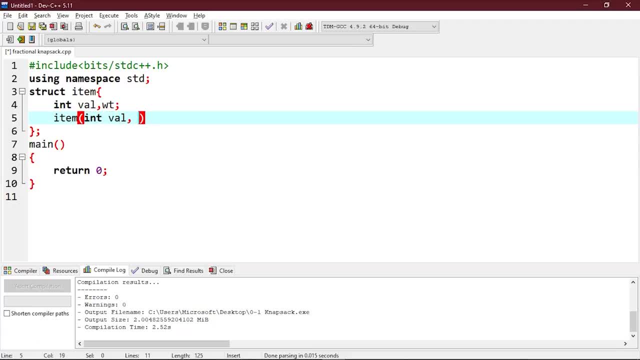 as int, val, comma, int wtVal, where this value will be equals to val and this weight will be equals to weight. Now we will write a comparison function to sort items according to value by weight ratio, So boolean function, cmp, With argument as: struct item a, comma, struct item b. 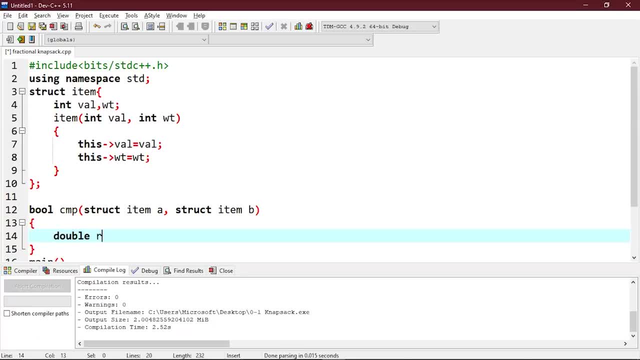 Now, double r1 is equals to double a dot value divided by double. a dot value divided by double. double a dot weight. Similarly, we will write it double r2, which will be equals to double b dot value divided by double a dot value divided by double. 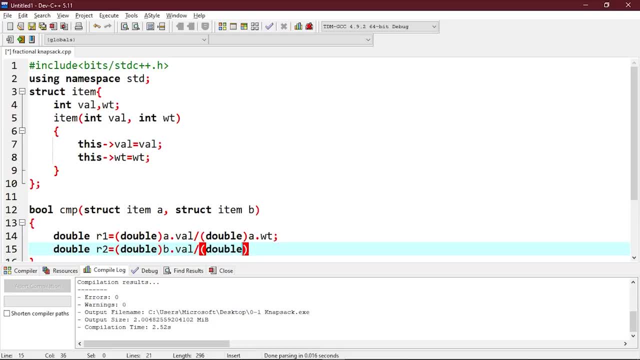 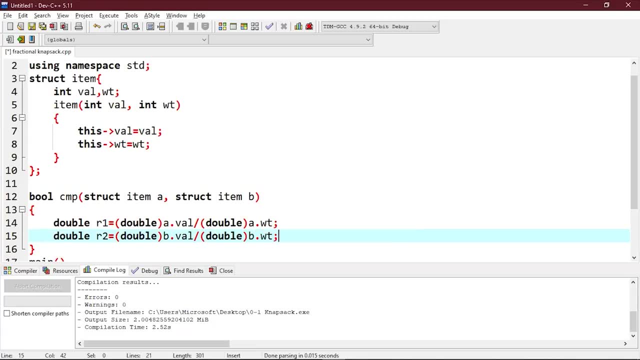 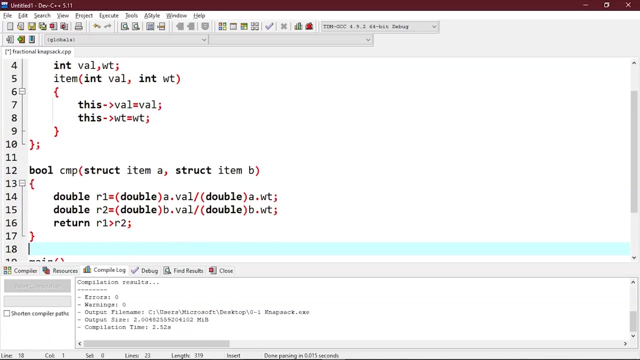 a dot weight. Now we will return r1, r2, or we will write: r2 will give us value above c Now, which means it will return true if r1 is greater than r2.. Now we will write the main function to solve the problem. 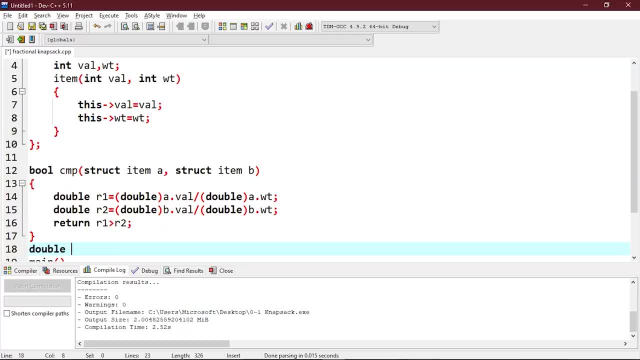 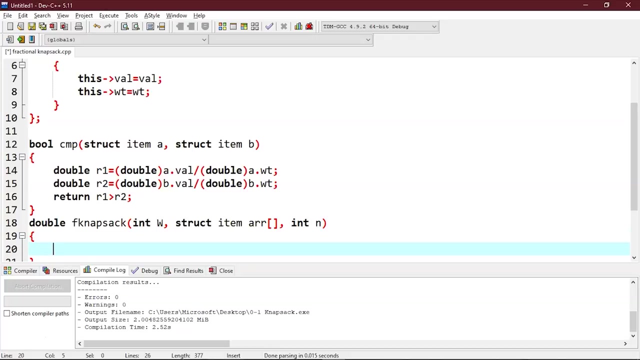 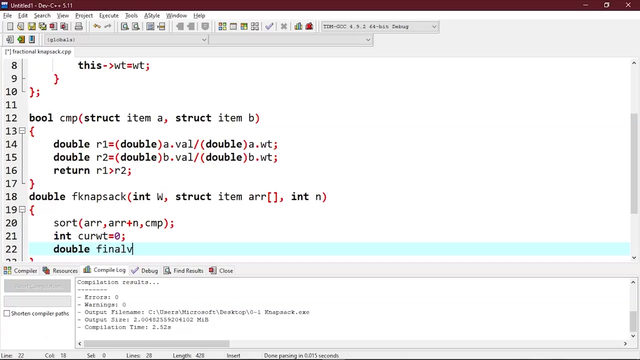 So double fNapSec with argument as int capital W comma struct, item arr comma int n. We will first sort the item on the basis of ratio. So sort arr comma arr plus n comma cmp. Now int current weight is equal to zero and double final value is equal to 0.0. 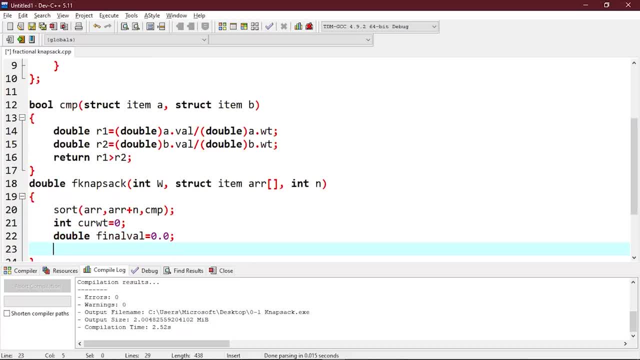 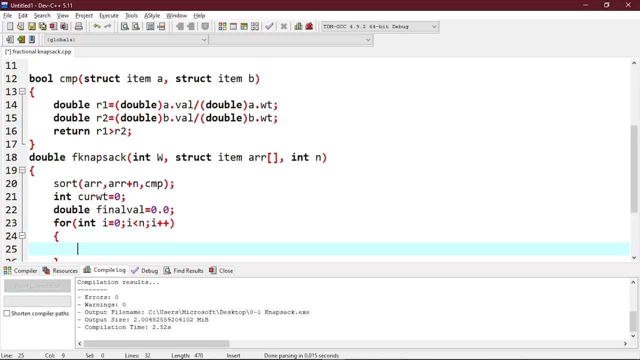 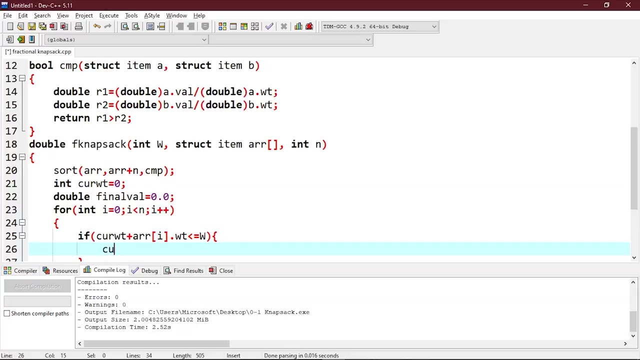 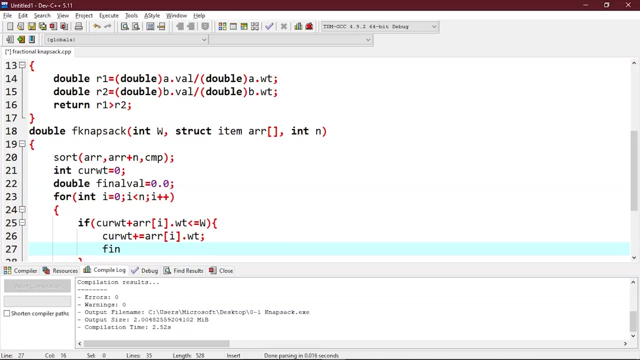 This will be result value in knapsack. So for, So for, For, For, For, for, for. for current weight plus ARR dot weight is less than equals to capital W, then current weight plus equals to ARR dot weight and final value will be plus equals to ARR dot value. 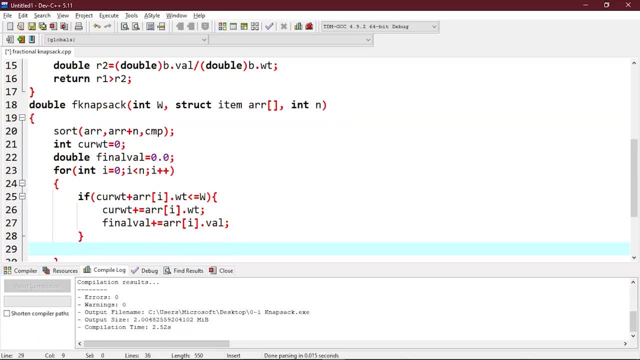 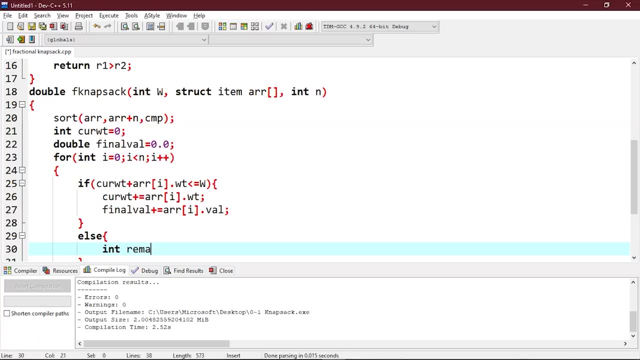 final value will be plus equals to ARR dot weight. now, if we can't add a current item, then we will add fractional part of it, so else now, if we can't add a current item, then we will add fractional part of it, so else int remain is equals to W minus current weight. 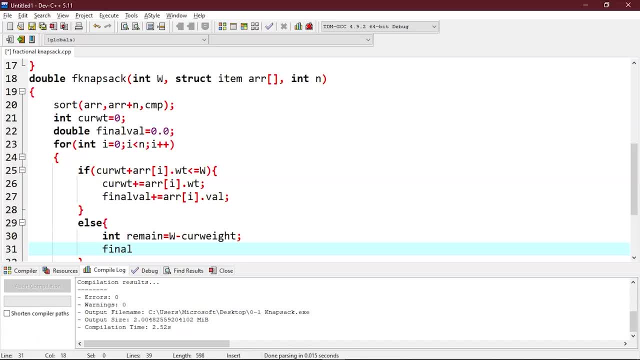 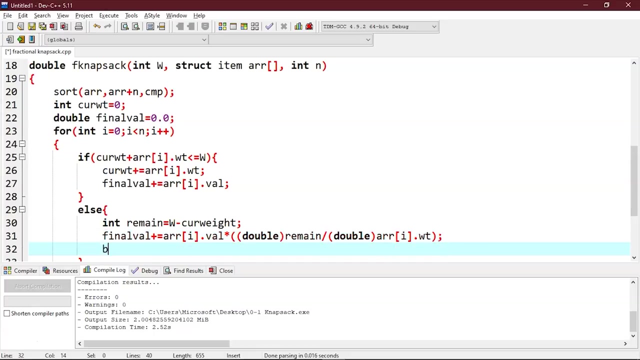 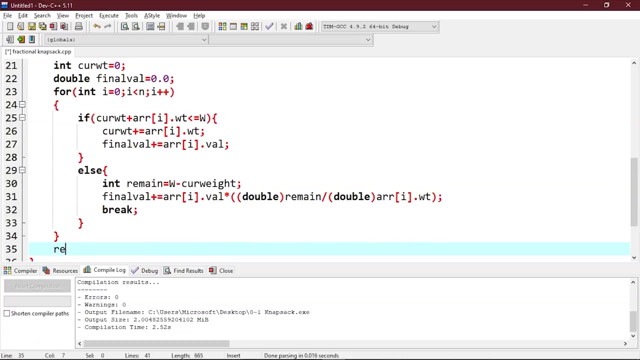 then final value will be plus equals to ARR dot value will be plus equals to ARR dot value multiplied by double remain divided by double ARRwait. now we will break, then we will return final value. now let's write our main block. we will start with defining int w equals to 50. 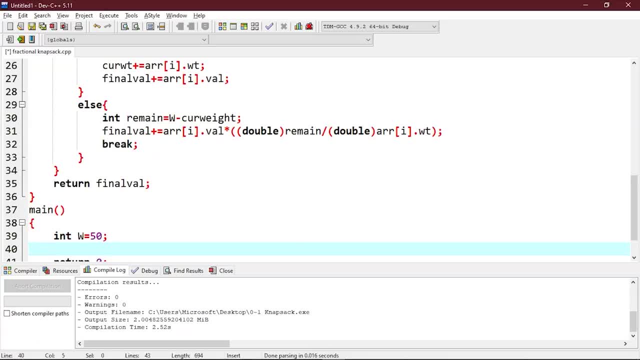 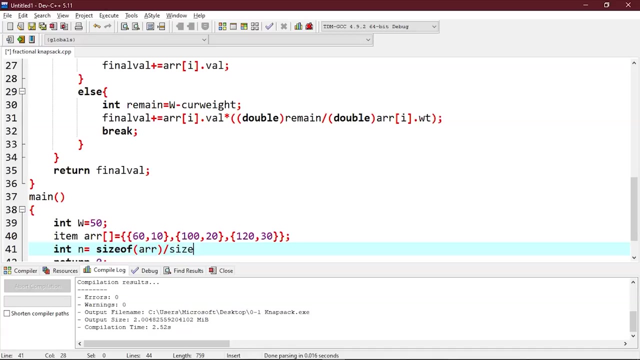 this will be weight of the knapsack and item. ARR equals to element. is 60 comma 10 comma, 100 comma 20 comma 120 comma 30. We will find the size of n and n equals to size of ARR divided by size of ARR at zeroth.